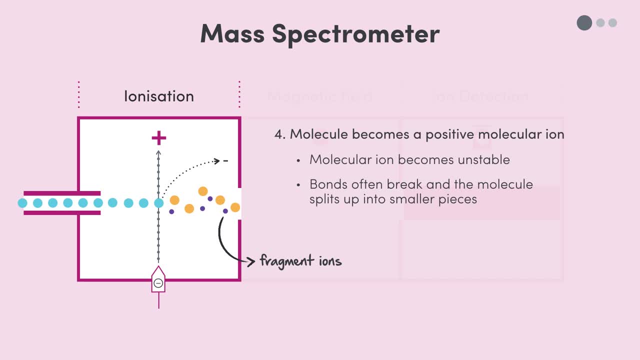 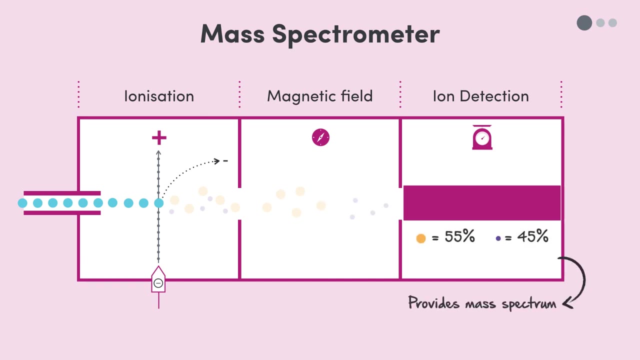 fragments or pieces of our big molecular ion. Fragment ions are separated by a magnetic field based on their mass to charge ratio or m over z. The number of ions with different m over z values are measured and compared by a detector, and voila, we get a mass spectrum. Now onto the 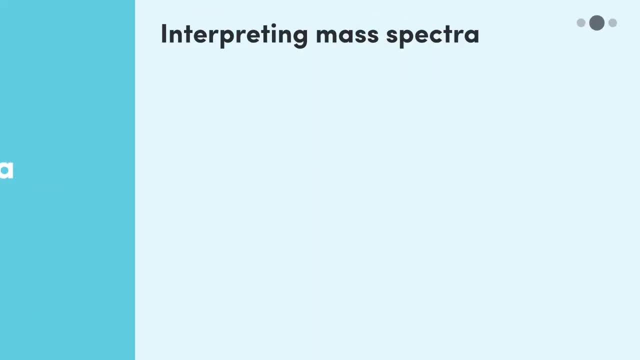 fundamentals of a mass spectrum which represents the results from our mass spectrometer. On the x-axis of our mass spectrum we have the mass to charge ratio, which is m over z, meaning mass divided by charge of the ion. Here, on the y-axis, we display the relative abundance. 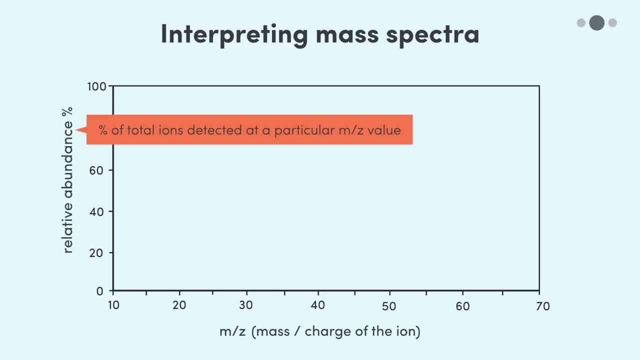 This is the proportion of the total ions detected that were recorded at a particular m over z value, and this is often given as a percentage. The peak with the biggest mass to charge ratio on our spectrum belongs to the molecular ion, so we call this the molecular ion peak. 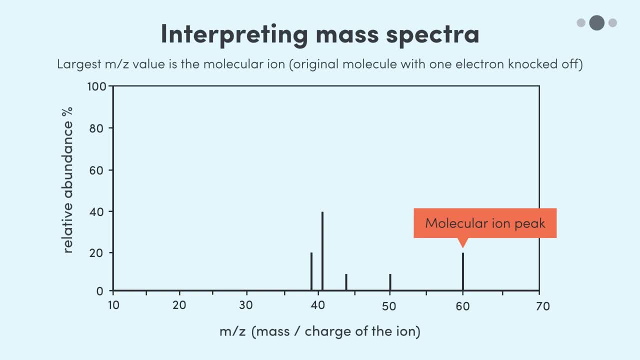 The molecular ion is basically the molecule being analysed, with one electron knocked off, making it the biggest complete molecule in our sample. This peak, which is the biggest peak in our spectrum, is called the base peak, and it represents the most abundant fragment ion in the sample. As a rule, the base peak is given a relative abundance of 100%, so 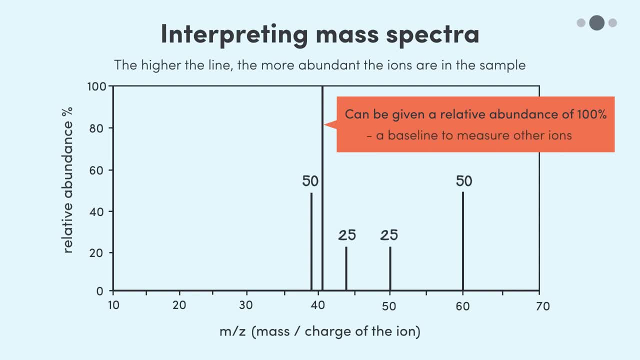 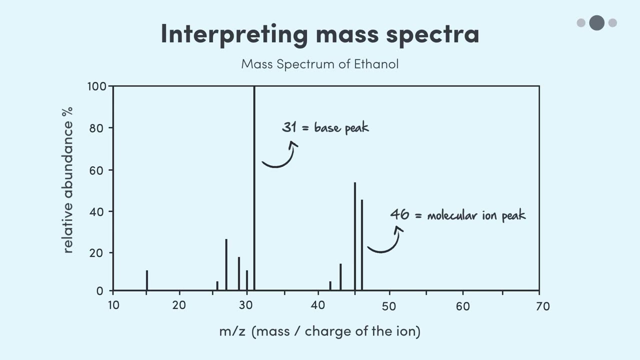 the abundance of all the other peaks are measured relative to the base peak. Using all this information, let's quickly look at a mass spectrum. We can see at the highest mass charge value of 46,. we have our molecular ion peak At a mass overcharge value of 31,. we have our base peak as it has the highest abundance. 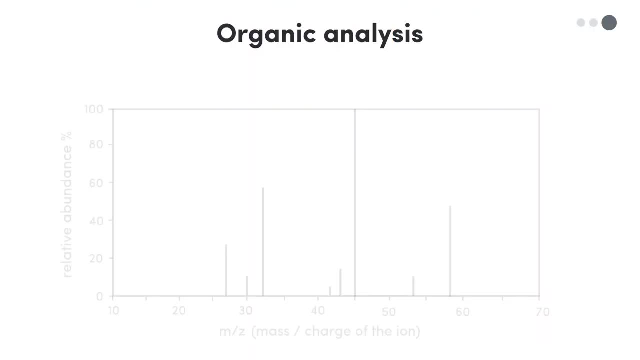 When we're using mass spectrometry for organic analysis, it's the molecular ion peak we're interested in, Because every molecule has its own unique mass spectrum. the molecular ion peak can help us to determine the identity of organic compounds by giving us information about their 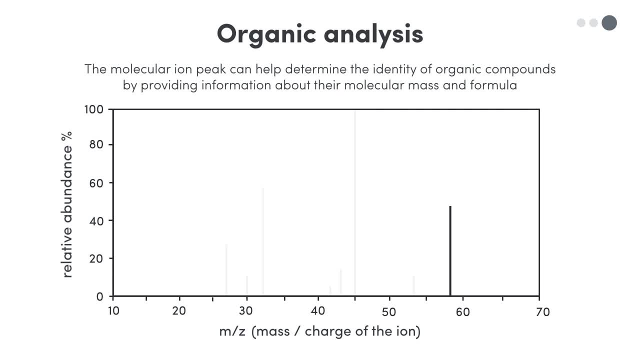 molecular mass and function. Let's look at an example to see how this can help us identify our molecular ion peak. You'll remember that the molecular ion is the biggest complete molecule in our sample and is formed when the entire molecule loses one electron. By losing one electron, the 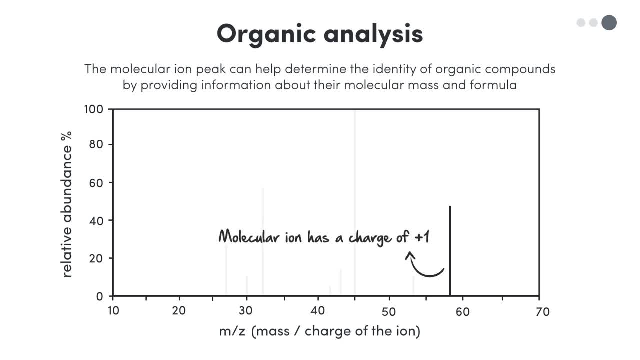 molecular ion has a charge of plus one. This means z, or the charge in our m over z value is equal to one. So the m over z value of our molecular ion is actually equal to the molecular mass of the molecule being analysed. Let's look at an example to see how this can. 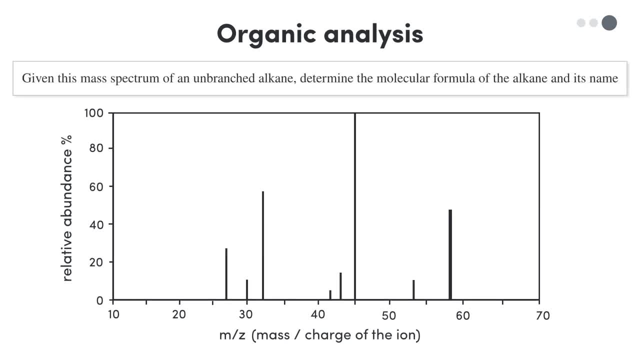 help us identify organic molecules. Given this mass spectrum of an unbranched alkane, determine the molecular formula of the alkane and its name. First things first, we need to identify our molecular ion peak, which is the peak with the highest m over z value. 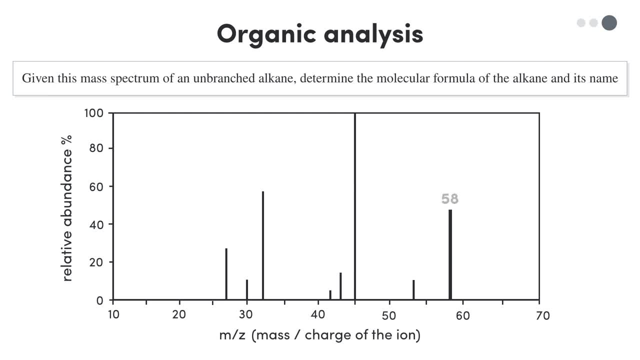 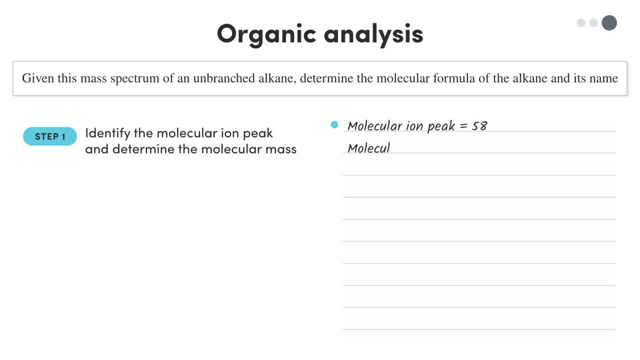 In this example our molecular ion peak has an m over z value of 58. We know this is equal to the molecular mass of the organic molecule being analysed. So our alkane being analysed has a molecular mass of 58. Next we write out the general formula of an alkane and, with a little organic chemistry, 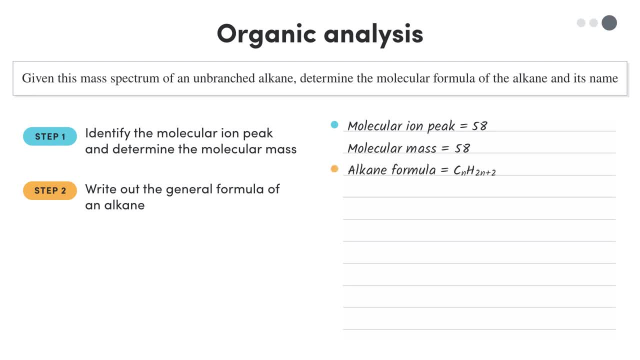 under our belts. we know that this is CnH2n plus 2.. Now, using this general formula, we have to calculate molecular mass. We know that the relative molecular mass of 58 is equal to the sum of the relative atomic masses of the atoms present in our alkane. 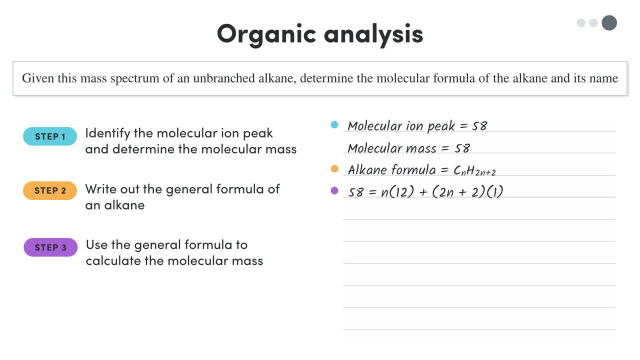 But we don't know how many of each atom is present. So we write an equation out like this and sub in our atomic masses. A little trick here: you should use the atomic masses of the most common isotopes of carbon and hydrogen- 12 and 1, rather than the relative atomic masses. 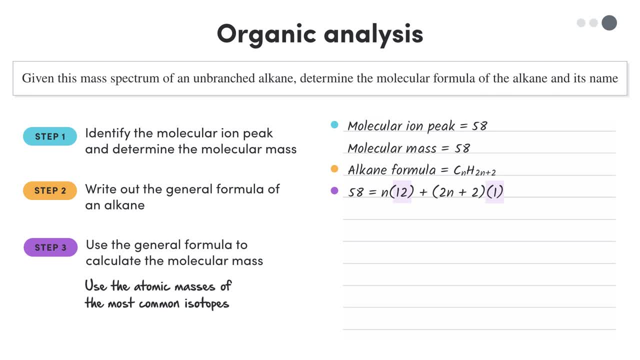 This is because the peak is produced by a molecule of the alkane containing only these isotopes. So 58 equals n times 12 plus 2n plus 2 times 1.. Then we solve for n and get 4.. So 58 equals n times 12 plus 2n plus 2 times 1.. 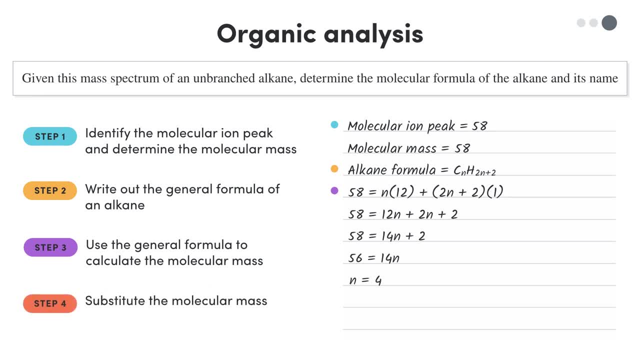 Then we solve for n and get 4.. Then we solve for n and get 4.. Now we can write out the molecular formula for our alkane. We substitute our value n equals 4, into the general formula for an alkane. 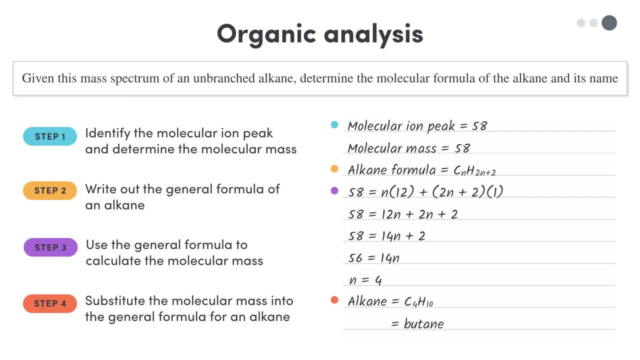 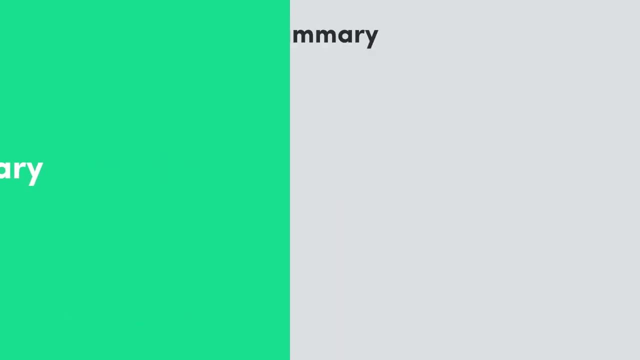 This gives us the molecular formula C4H10 and tells us our alkane is butane. And that's it for this video. everyone. Just a few key points to remember. Mass spectrometry is a quantitative analysis technique that can be used to identify and. 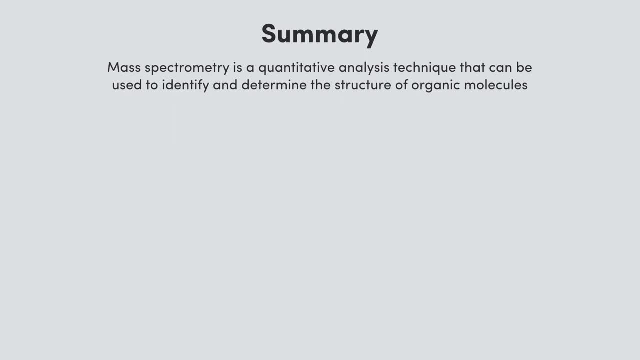 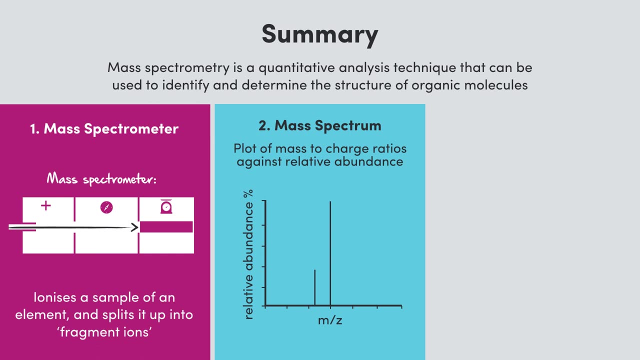 determine the structure of organic molecules. In this video, we looked at how to identify the structure of organic molecules. We looked at how to identify organic molecules using a mass spectrum, which is a plot of the mass-to-charge ratios of the ions produced by ionising our sample and the relative abundance.